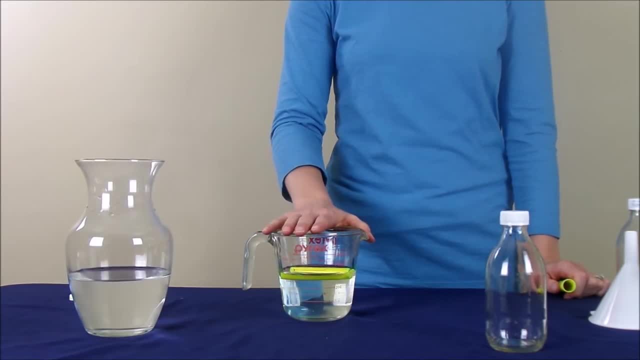 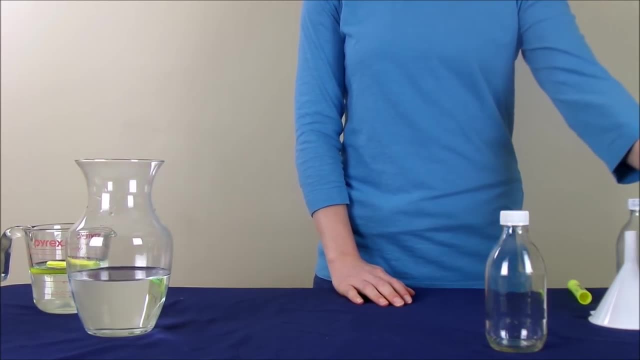 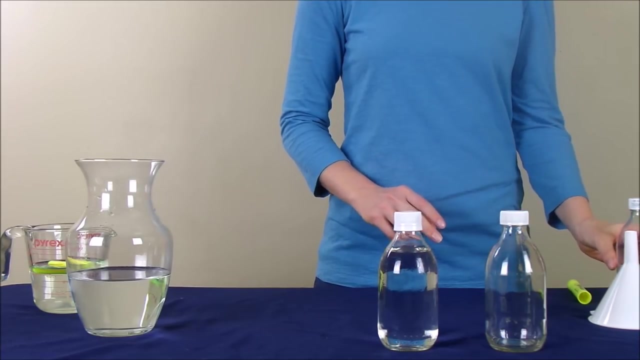 into the water And we're going to let it sit for a little while. The second bottle of water is going to be some tonic water, And this is just regular tonic water that I purchased at the store, And then the last bottle of water is going to be some water. 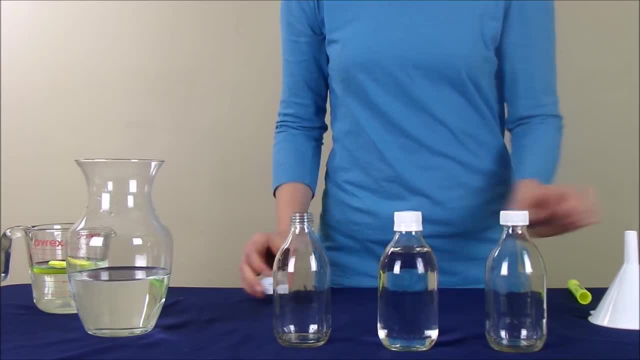 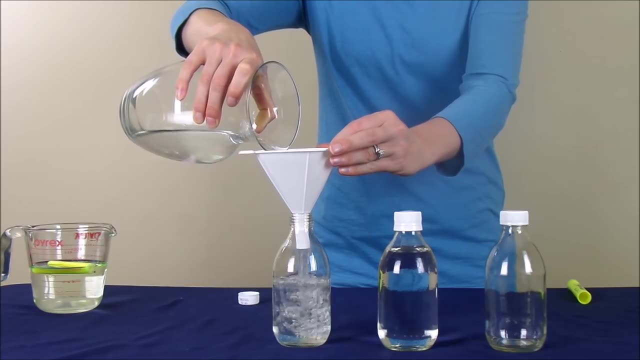 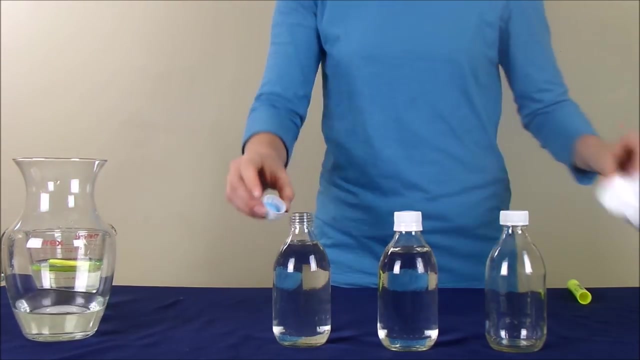 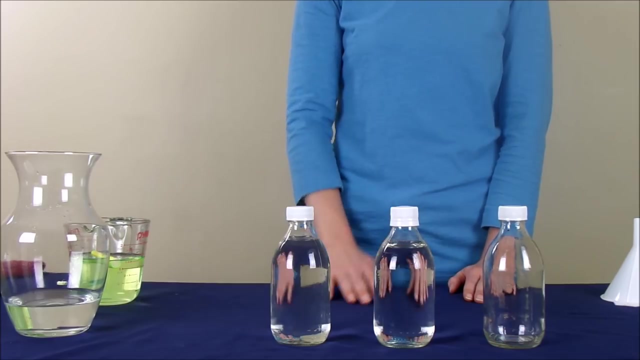 that is just going to be regular water, So I am going to fill the bottle up using my funnel. So, now that the last two bottles are prepared, we are going to check on our dyed water, We are going to take this and we are going. 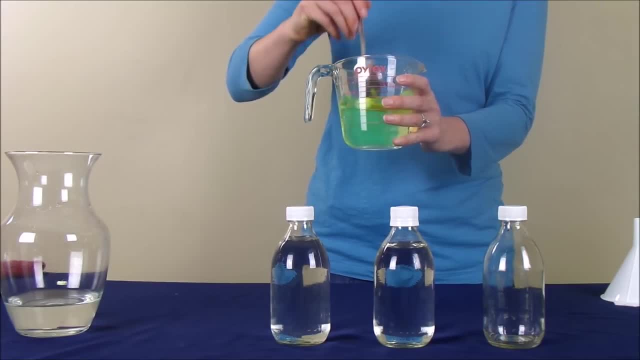 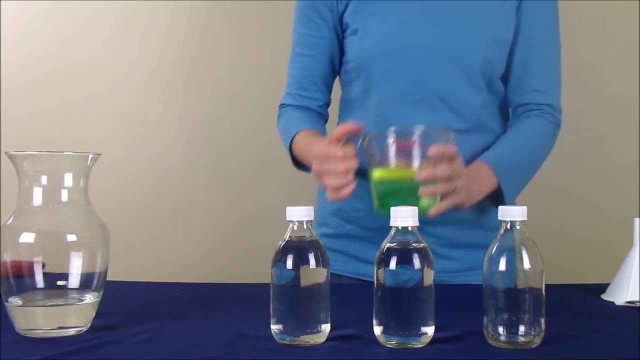 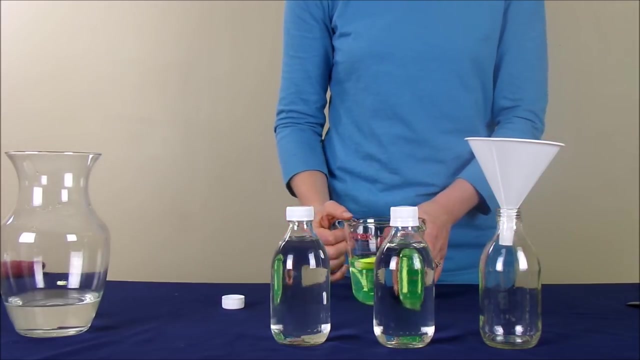 to take a spoon and just kind of stir it up just to get the the last of that ink into the water. Then we're going to take that first bottle. it's still empty and we are going to pour our dyed water in it. 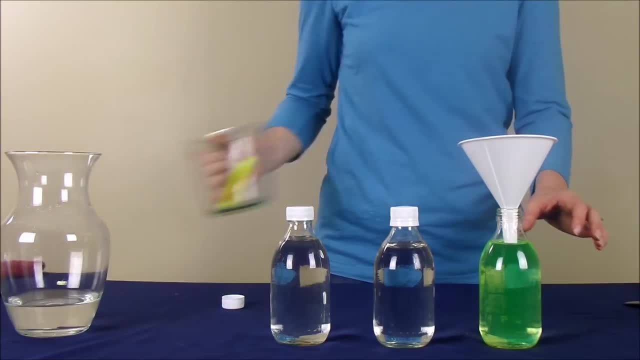 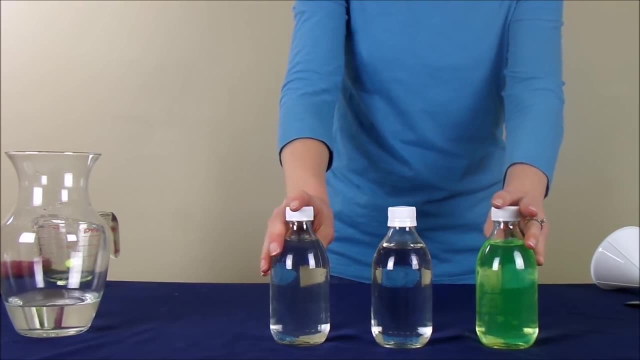 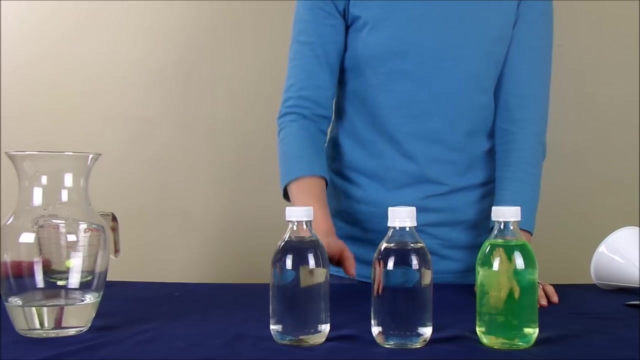 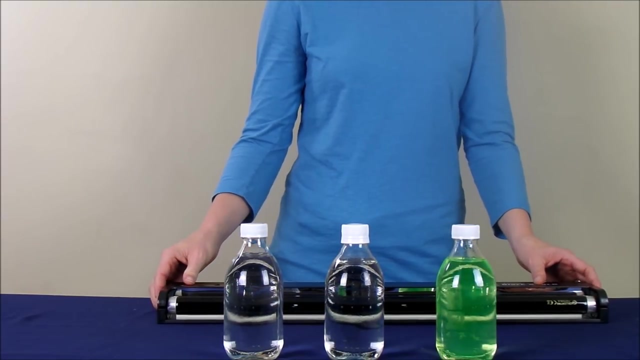 So now we have our three types of water. We have the dyed water, the seltzer water and the regular water. Now for the next step. you should position your black light next to your bottles. Then we're going to turn out the lights and turn the black light on. 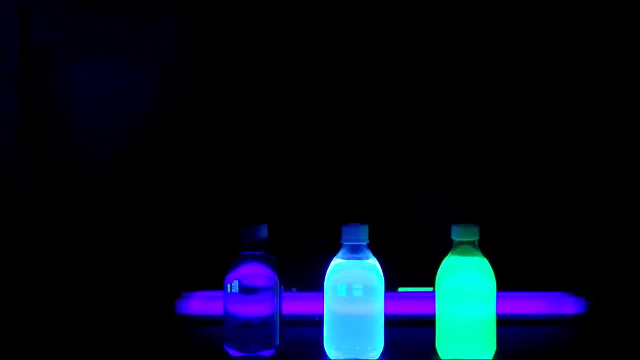 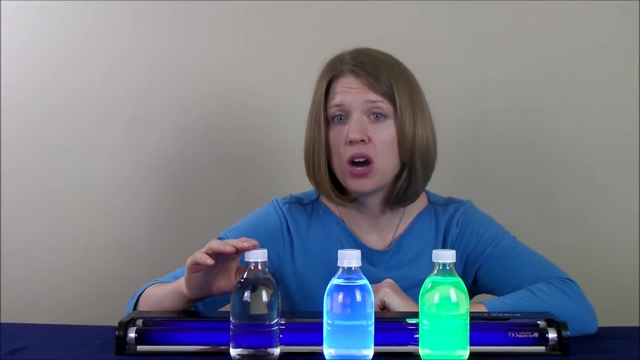 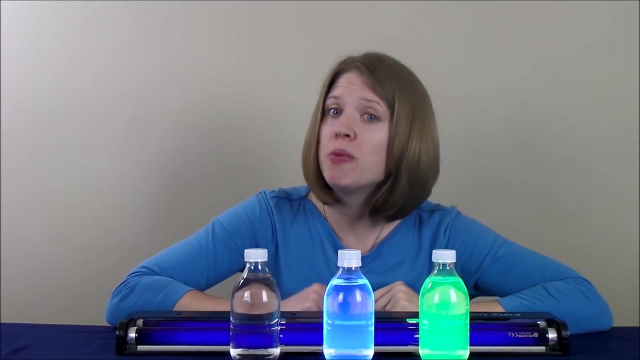 So, as you can see, the regular water does not glow, the dyed water does glow, and so does the tonic water. So can you tell me why that happens? Leave a comment below to submit your guess and then visit CoolScienceExperimentsHeadquarterscom to find out why. 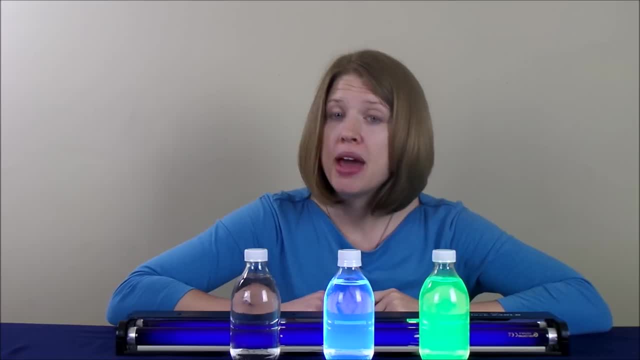 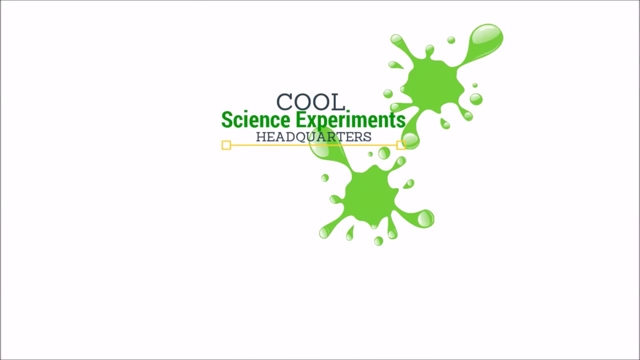 You can print out detailed instructions for this experiment, and you'll find many other cool science experiments at CoolScienceExperimentsHeadquarterscom. There are many more experiments that you can do at home too. Thanks for watching everyone, and we'll see you next time.